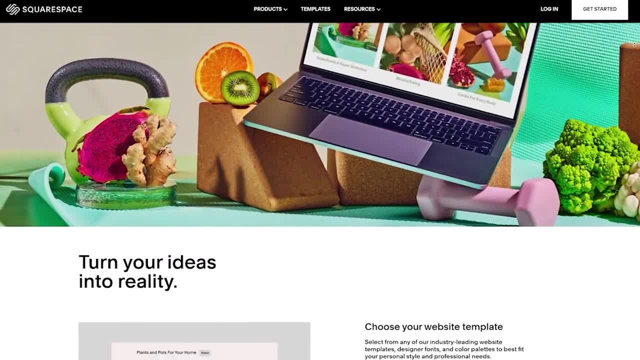 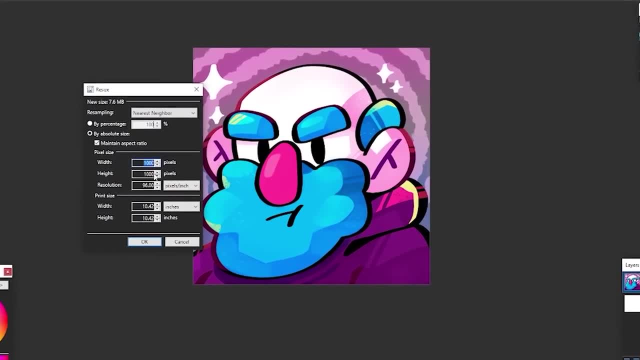 Believe me, I've done it many times before And the best way to cut the hassle is to use Squarespace From selling your products online, making a portfolio or gallery of your work, or even something as tedious as image scaling. it's so much easier and saves you so much time with Squarespace. 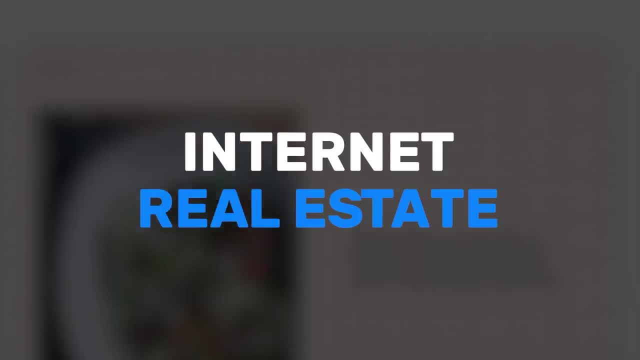 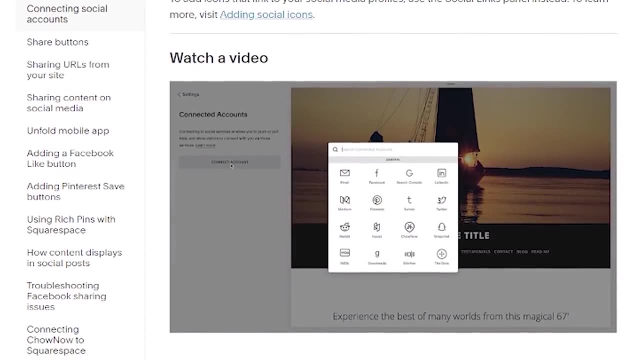 As the internet expands, I truly believe that everyone should have internet real estate. But creating your own website doesn't mean you have to be disconnected from social media. With Squarespace, you can connect your social profiles, so that way you can instantly post on different platforms. 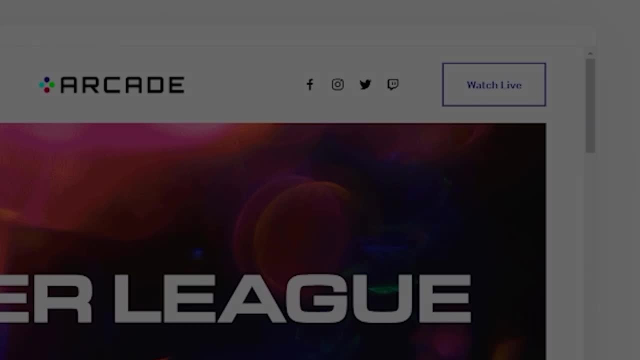 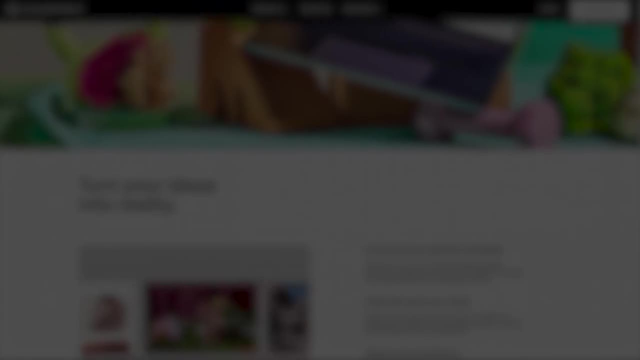 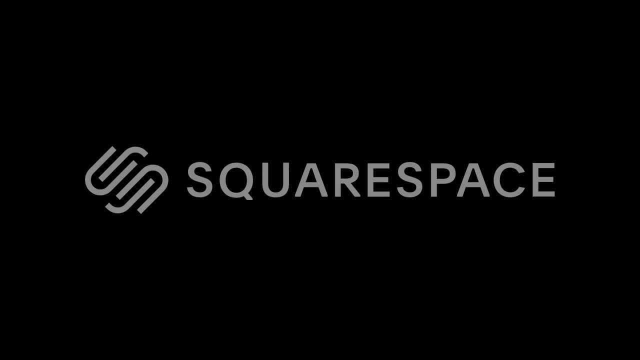 making it fantastic and easy to post your new product or game. Make sure to go check out squarespacecom for a free trial And when you're ready, you're all set to launch. go to squarespacecom- goodguess, to save 10% off your first purchase of a website or domain. 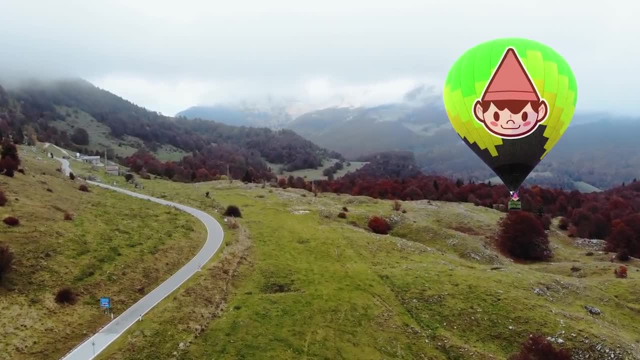 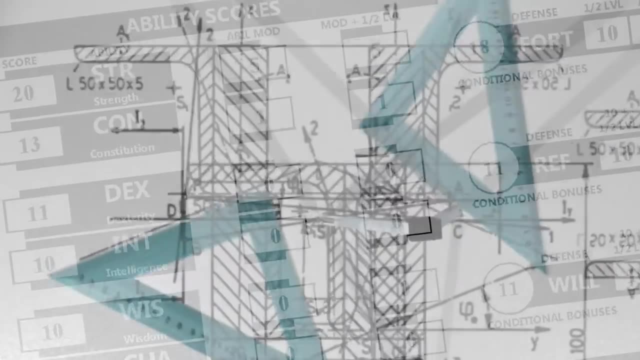 Now, before we get ahead of ourselves, it's probably best to explain why I wanted to make my own game in the first place. You see, most tabletop role-playing games are like reading scientific journals: They're full of insanely detailed characters with complex mechanics. 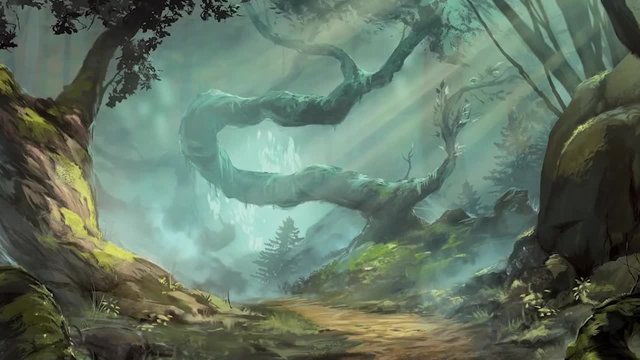 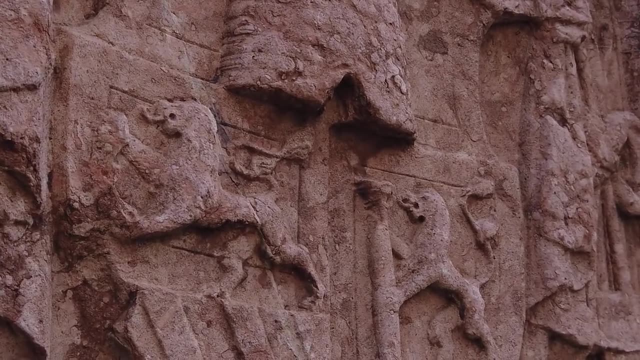 and long drawn out backstories, And for some people that's what they love about it. They love the details, they love the complexity, But for me, the appeal of a tabletop game came from the creativity and the imagination. I love the idea that I could sit down with my friends and we could go to this world. 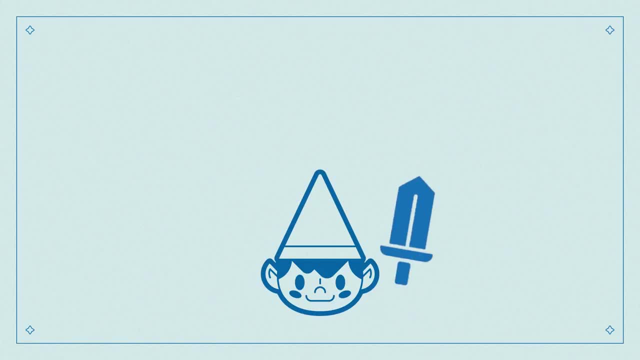 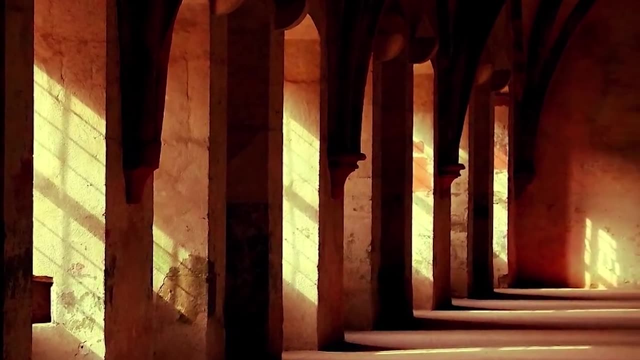 in our imagination together and have a fun adventure, kick some monster's butt and then call it a day. I also like adding a lot of humor to my games, because I just feel like all adventures should have some sort of funny moment, Unlike some role-playing games which can be really depressing and serious. 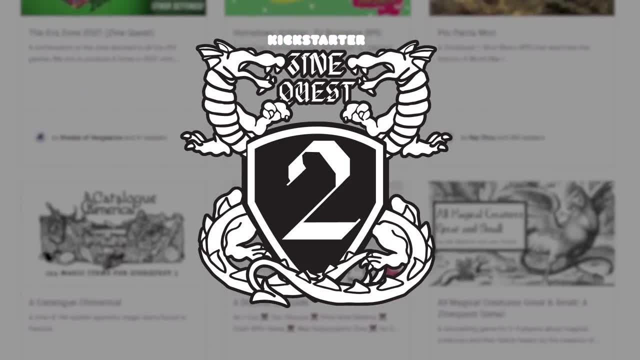 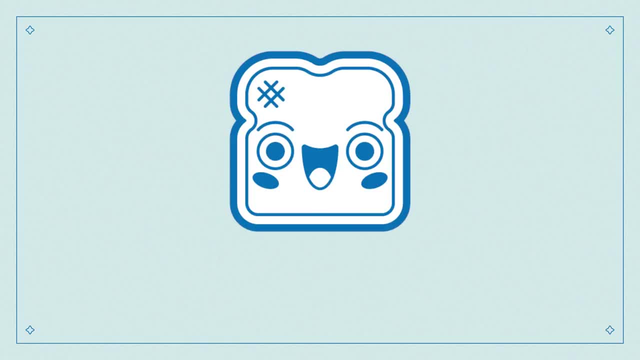 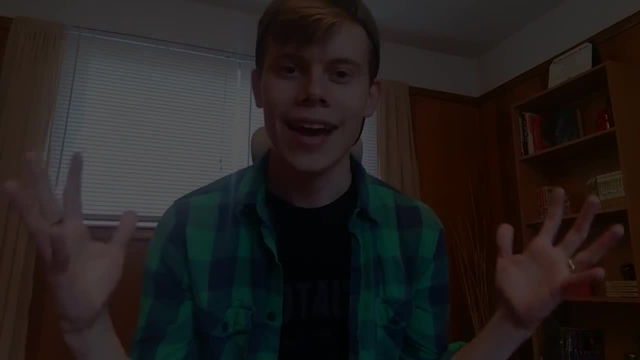 and it just feels too stuffy. So after seeing ZineQuest, I knew I had to make a game and I couldn't do it alone. So I recruited my close friend and fellow graphic designer, Brad, to help me out. So, with optimism in our hearts and a twinkle in our eye, we began creating Snohms. 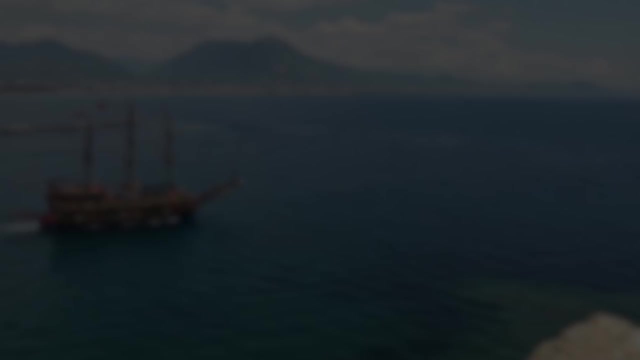 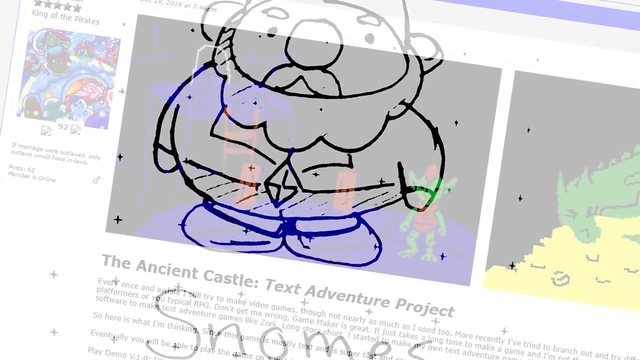 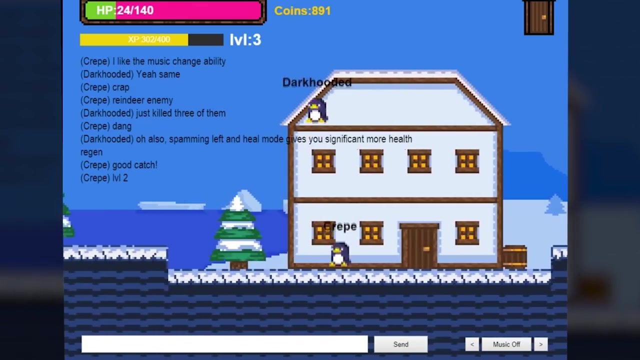 Now to say that I started from a completely empty slate is probably unfair. I actually created Snohms a couple years prior, before I started Feareth. It was for this winter Christmas form website we made. The website's whole purpose was to challenge us to make winter creative things. 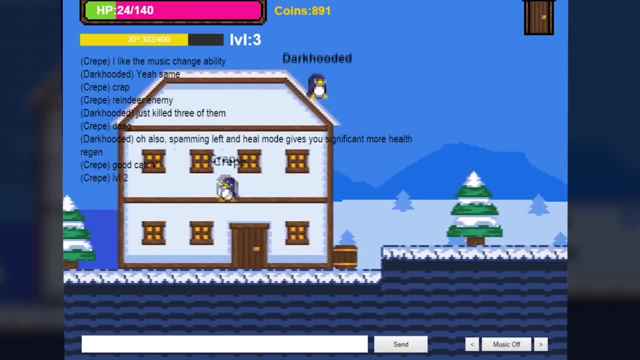 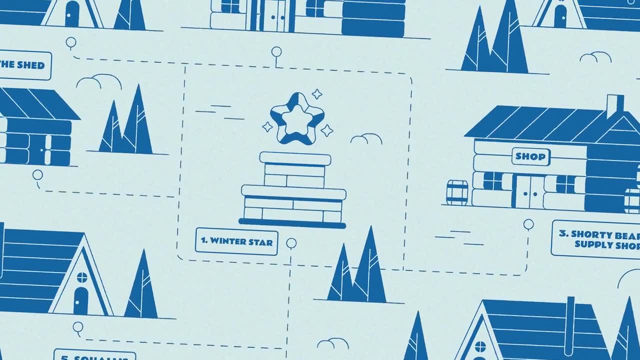 It could be movies, It could be stories- Super random- But one of the ideas was about this town that was going to freeze over by Christmas And the people on the forum had to comment. They had to figure out the mystery of what happened to this winter star. 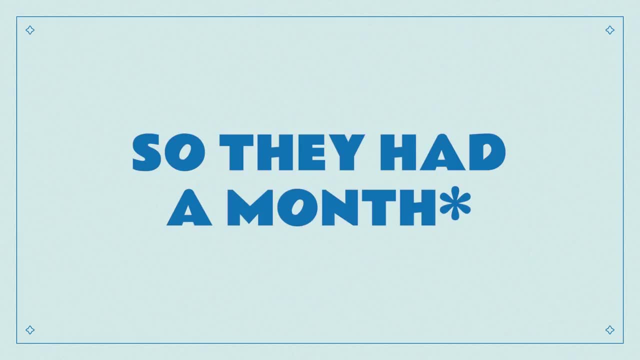 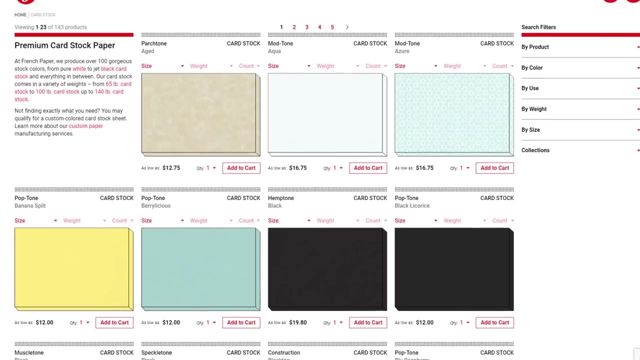 and save it before Christmas happened, So they had about a week in real time. Now I wrote a lot of detail about the characters in the town and the story. So, already having an idea, we figured out how we were going to print and manufacture the booklets. 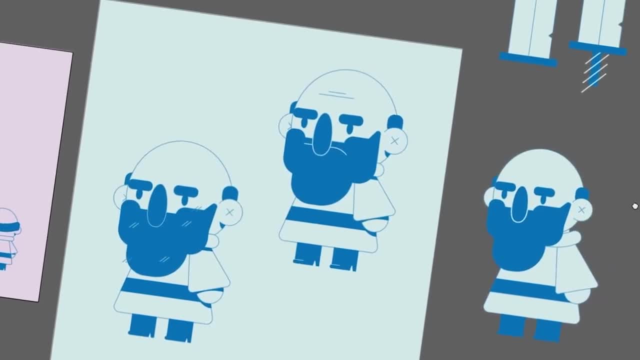 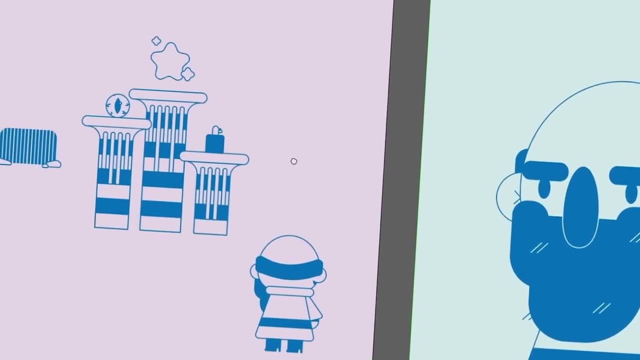 And then we just came up with some concept art. One of the main goals I had for this zine was to just push my self to try something different, So I wanted to illustrate in a style that I had never done before. Eventually, Brad and I bounced a couple ideas back and forth. 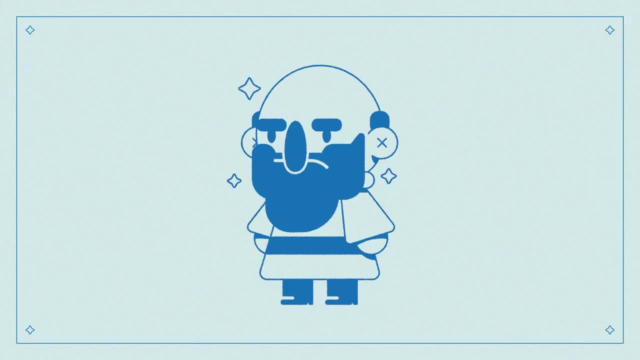 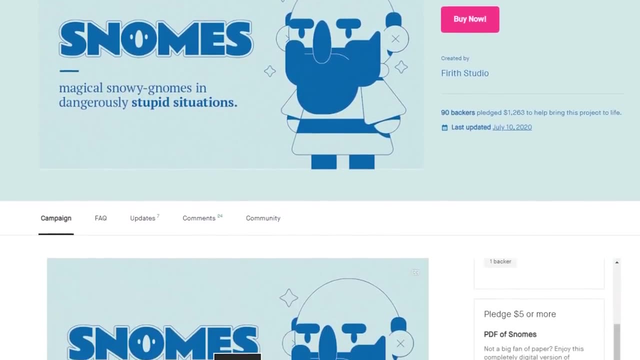 until we ended up with this lovely Snohm artwork. But then we made a huge mistake, Releasing the kickstarter before the game was finished. We knew that zine quest was about to start and we didn't have time to fully flesh out and write the copy for the game. 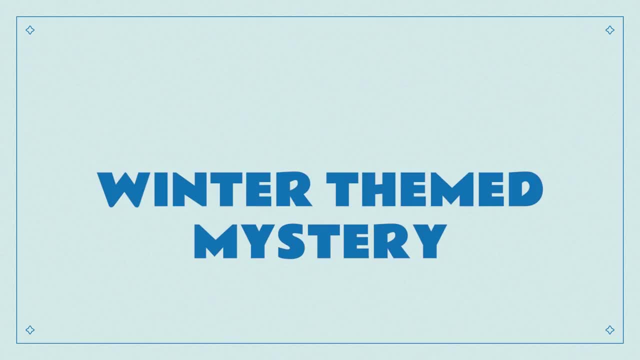 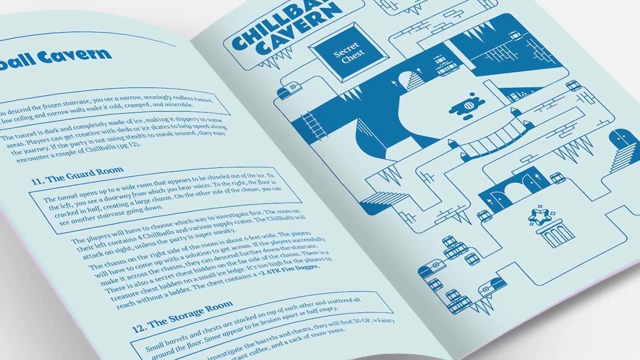 So we quickly came up with the concept behind the game. We tested it. once We created the character, We created the character sheet, a map and the Snohm illustration. That's all we had. 90% of the book was not complete. 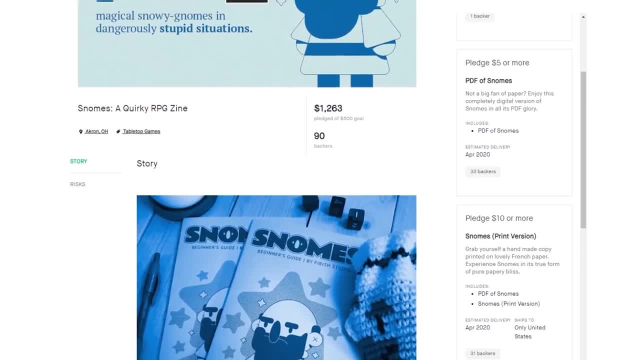 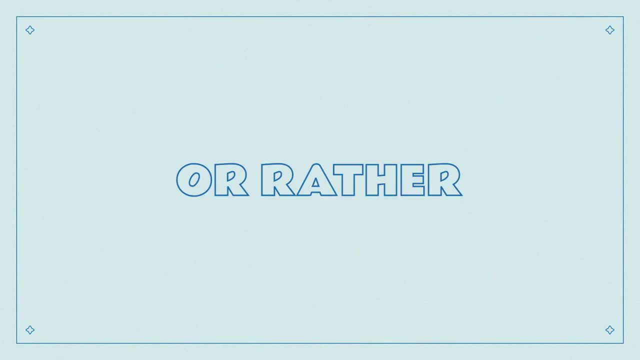 But we ran out of time and we decided to launch the kickstarter anyway And, to our surprise, it actually turned out really well. Now, I never explained the main gimmick or the main mechanic of Snohms, And the main mechanic is that you play as these magical winter gnomes. 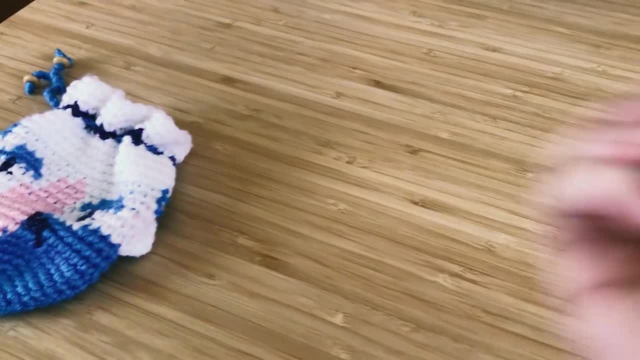 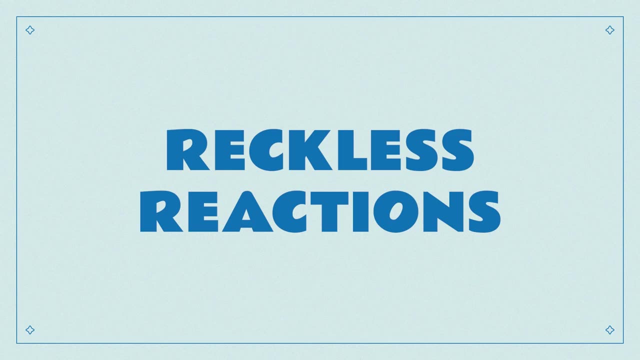 that are self-proclaimed masters of magic And basically whenever you roll a one on the dice, something terrible is about to happen, And those are called reckless reactions. So it's these weird magic abilities- You actually get to pick them- that happen. 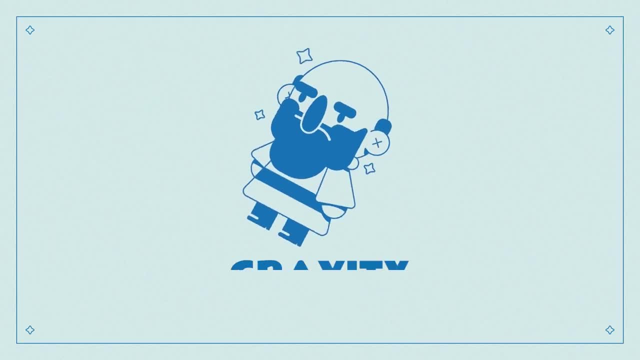 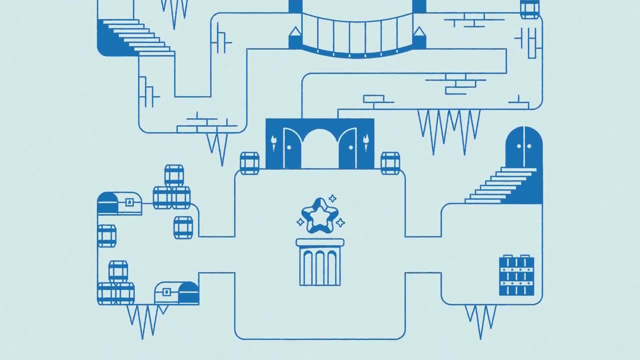 They can range from shooting a fireball out to gravity changing or even you turning into a lamp. Now, the game is meant to be extremely chaotic- And believe me, it is- And, if you love being a game master and running role-playing games, 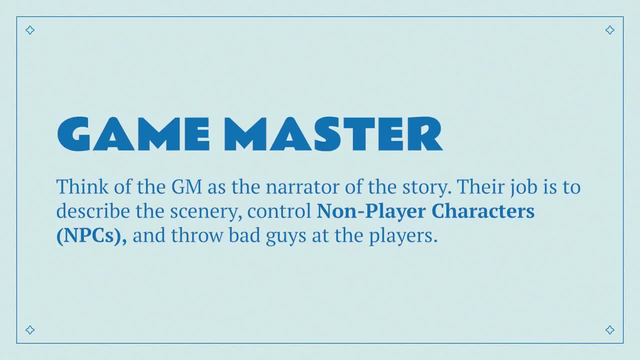 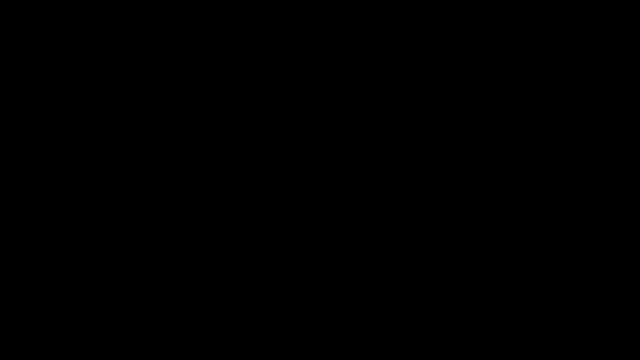 you'll find that this game really keeps you on your toes And you have to constantly be thinking about new ideas, thinking about new ideas and thinking about new ideas, And that's why we're going to keep the players from basically destroying themselves. 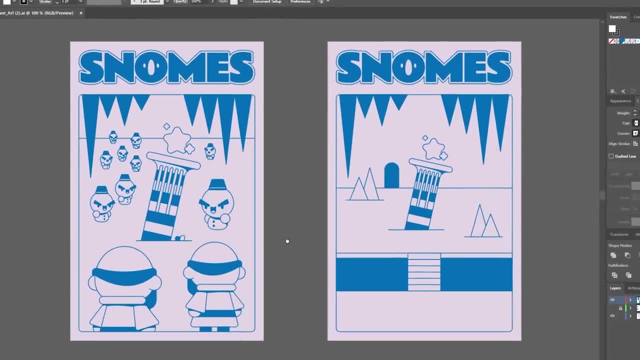 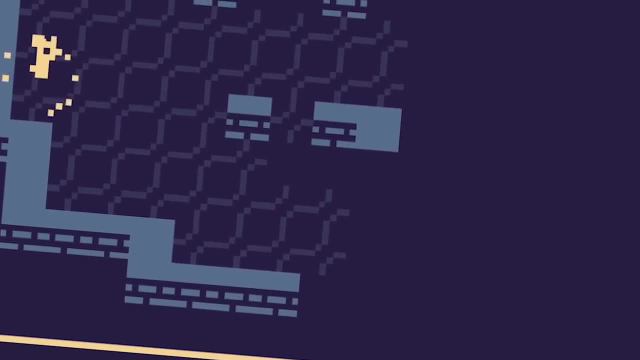 So once the kickstarter finished, we kind of relaxed. We felt good, We created this game and we did everything within two weeks, which is not that long of a time at all. But then we got busy, We got sidetracked. 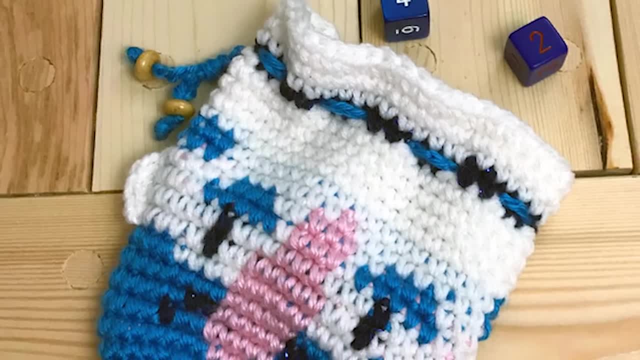 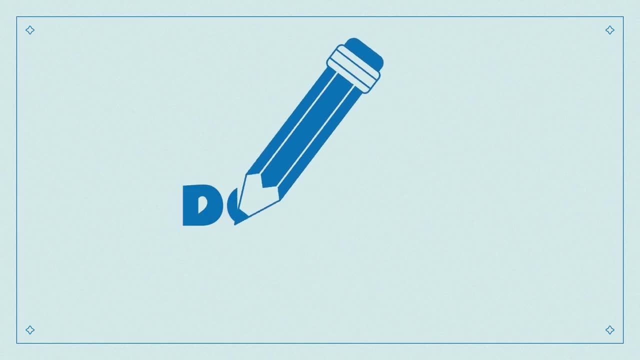 We had other projects that we were working on And, don't get me wrong, we did order the dice. We got everything set up that we needed in order for us to ship. It just was the writing portion. It's the sitting down to do it in the first place. 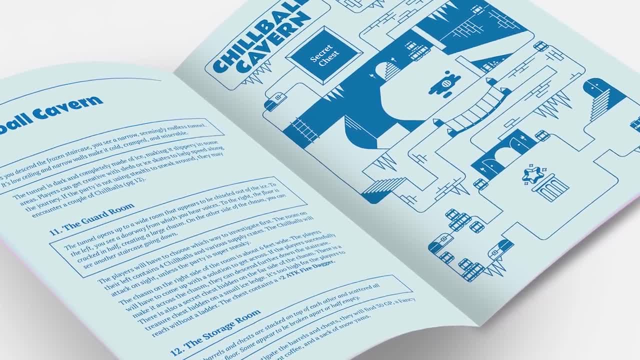 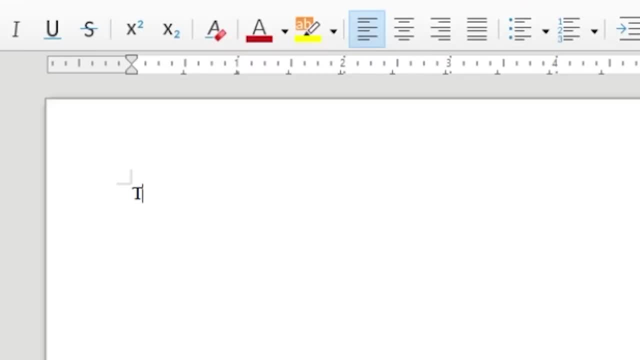 Especially a book that needed to be finished and published and sent out within a month. But the pressure of the kickstarter started to get to me And I was starting to get writer's block. I didn't really want to make anything, I just was super intimidated. 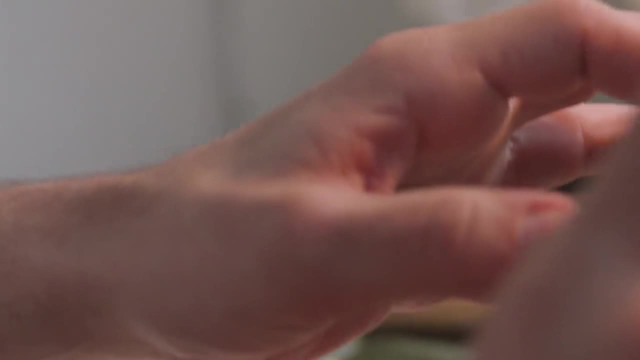 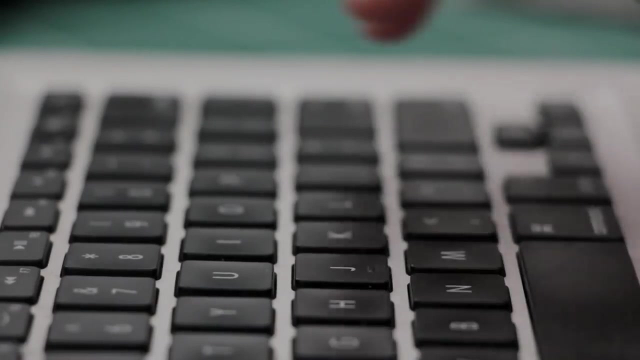 Until, finally, one day, I decided I was going to spend the week doing nothing but writing. I wouldn't talk with friends, I wouldn't get distracted, I wasn't even going to go outside, I just had to write. And so I wrote, every single day for hours. 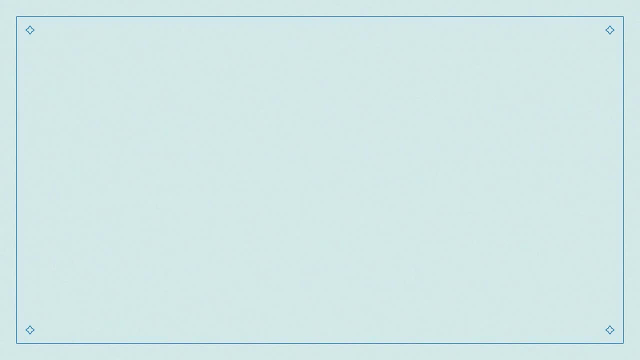 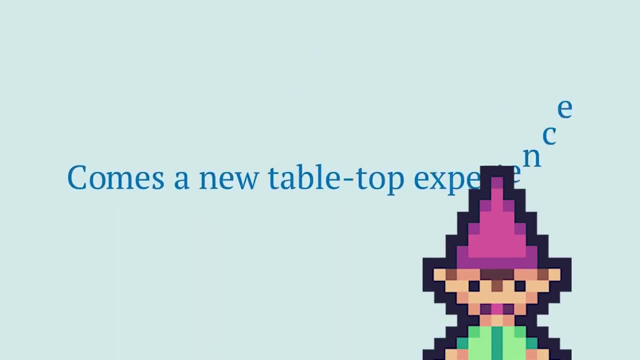 And I just was focused. I would think about it, I would think about the game, I would think about the concepts And when I would finish a page, I'd reach out to Brad and have him do an illustration. And after spending a week in isolation and focus, I finally finished the game. 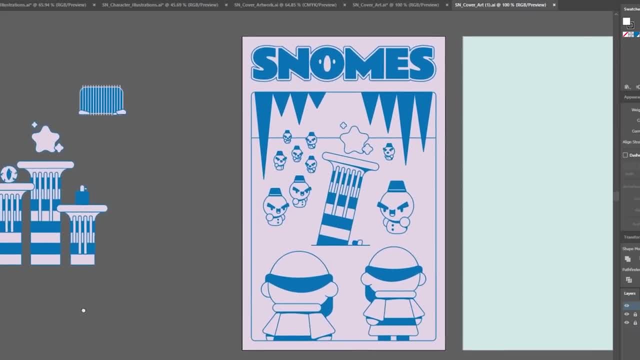 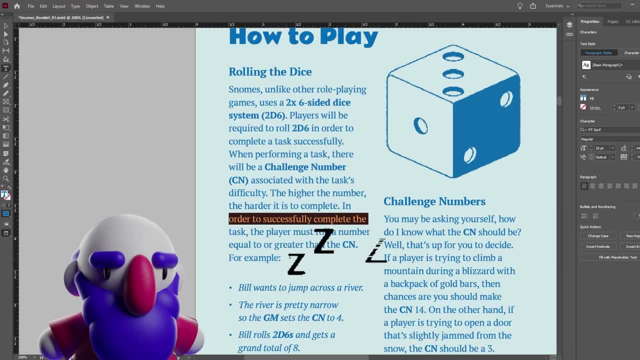 All that was left to do was the fun part: Creating more illustrations and doing all the typesetting. Now, I'm sure for a lot of you people out there at this point you're snoring Typesetting. How can that be fun? 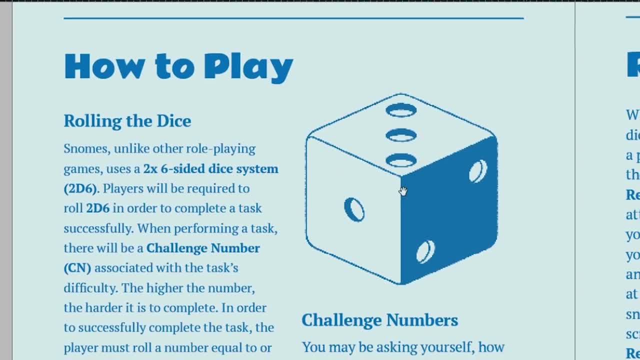 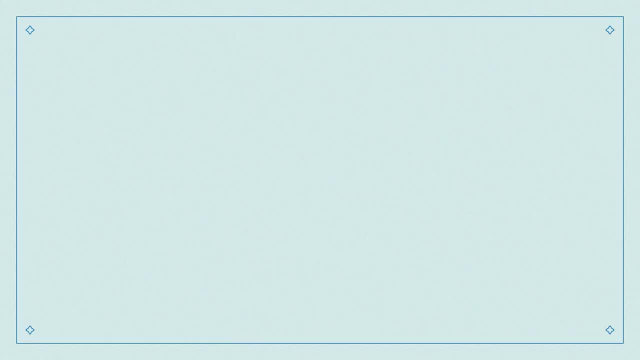 But there's something so satisfying by picking up fonts, laying out your book and just setting your type perfectly, And after I finished that, all that was left to do was to print the copies and send them off- And, luckily for me, Brad is a total chad when it comes towards printing and shipping things. 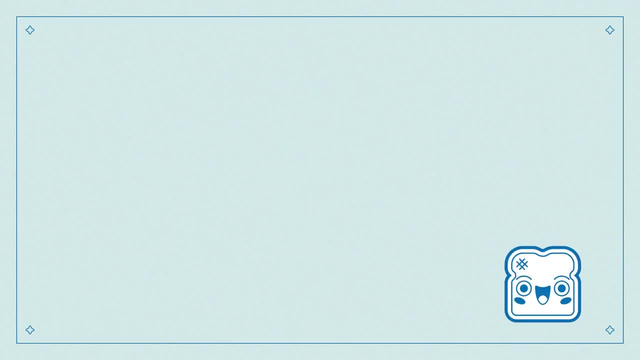 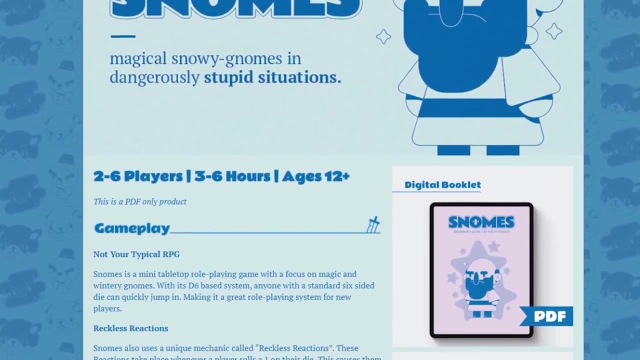 And he took care of all that with his lovely wife super fast. Now for those of you out there that actually want to play the game for yourselves, it's actually available on itchio right now. There's a print and play version. You can print it out and start playing with your friends. 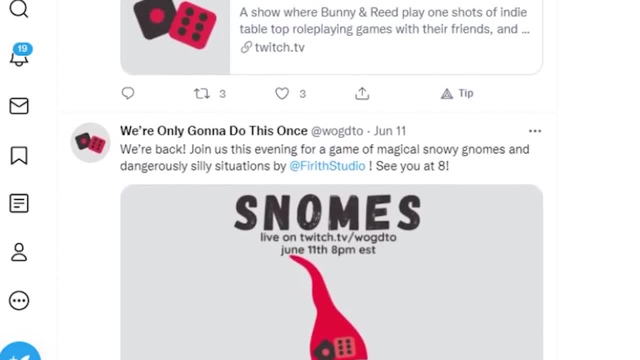 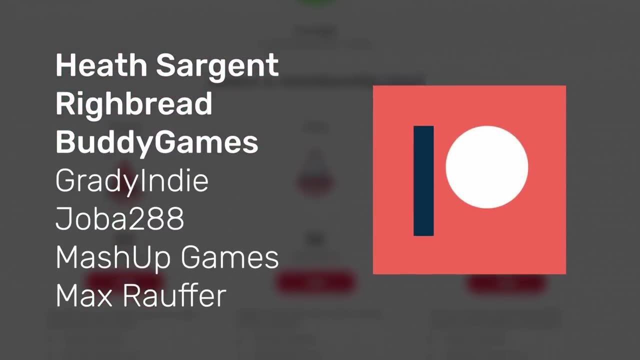 You can play it online. There actually was a group that live streamed it recently and it looked like they had a blast playing it. I just want to give a huge shout out to Heath Sargent, Rye Bread and Buddy Games and the rest of the fantastic Patreon supporters who make these videos possible. 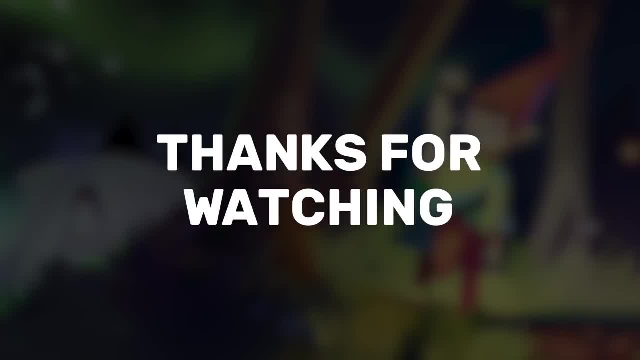 And I just want to thank you for watching. I hope you have a lovely rest of your day and I'll see you next time for another game dev adventure.